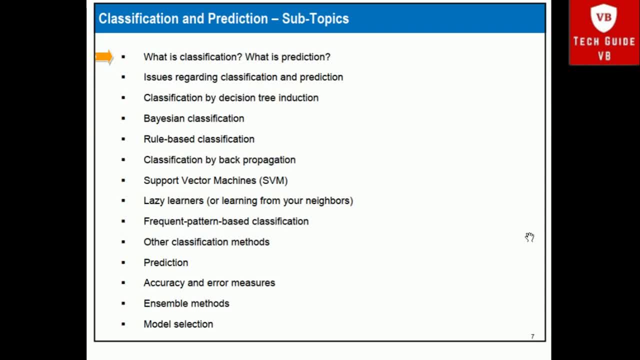 subscribe to channel for latest updates. so today's topic is classification- prediction. it is divided into number of subtopics, which we will cover in the further videos. so what is classification and what is prediction? that we will see first. then we will see issues regarding classification and prediction. then 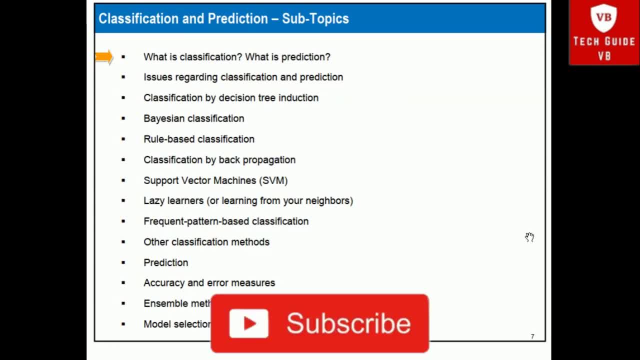 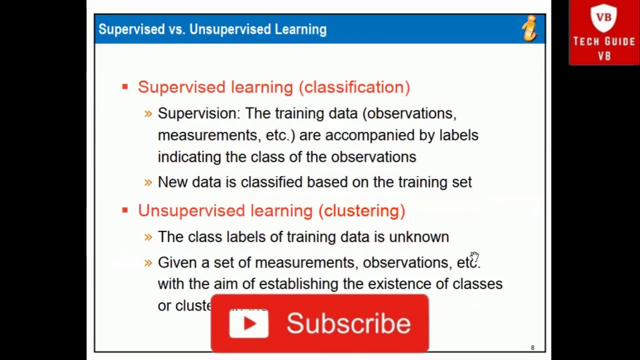 classification and prediction will be related to classification and prediction by decision tree induction. so this we will see in today's session. before going to start, what is classification and what is prediction? we need to know the difference between supervised and unsupervised learning. these two terms are new to you. that's why I will discuss this two term first. then we will see the. 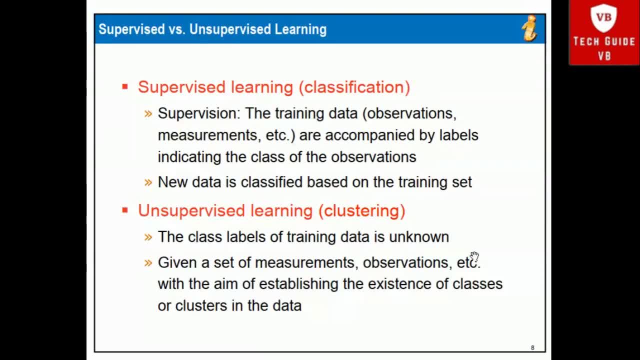 next part. supervised learning. in classification means what the training data are accompanied by labels indicating the class of observations. so there is a training provided to the given model in supervised learning. so in supervised learning we have the historical data set. according to that data set or according to the sample, we will train the model according to sample. 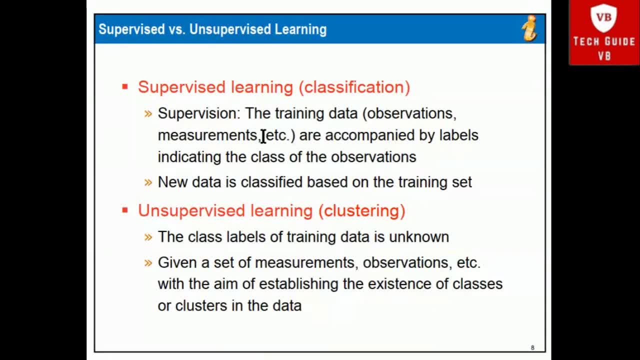 we will train the model and we will classify the label according to that. so the new data is classified based on the training set. so there is a training and testing. these two sets are there in supervised learning. so if new data comes, that data is classified based on the training set and in unsupervised. 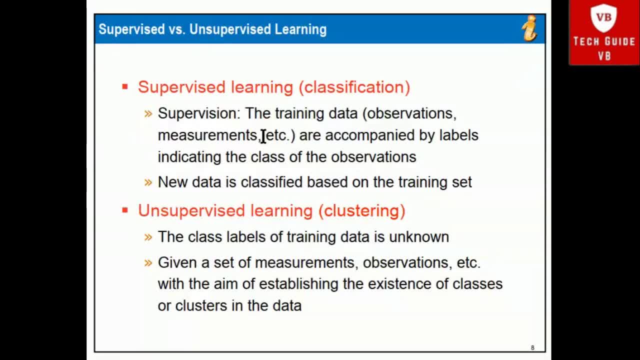 learning or in clustering. the class label of training data is unknown. there is no historical data present for the training. so, given a set of measurements, observation etc. with the aim of establishing the existence of classes or clusters in the data. so, according to the data, we will have the cluster and according to cluster, we 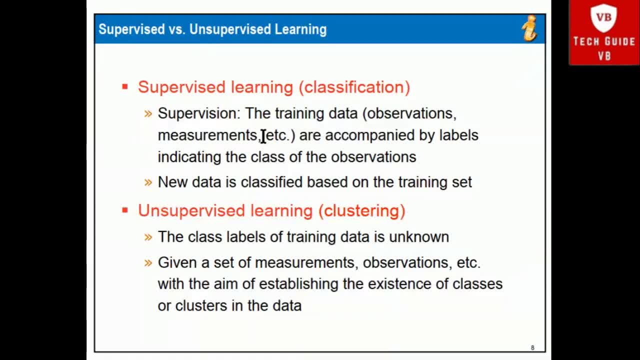 will do the operation. this is the unsupervised learning basic differences. in supervised learning, there is a historical data present for the training and an. in unsupervised learning, there is no such historical data present for the training, so supervised learning is basically used for the classification unsupervised. 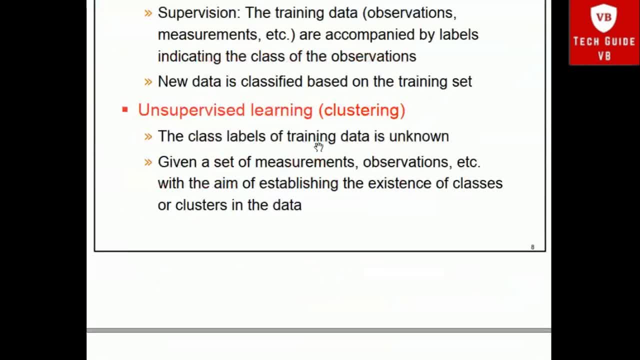 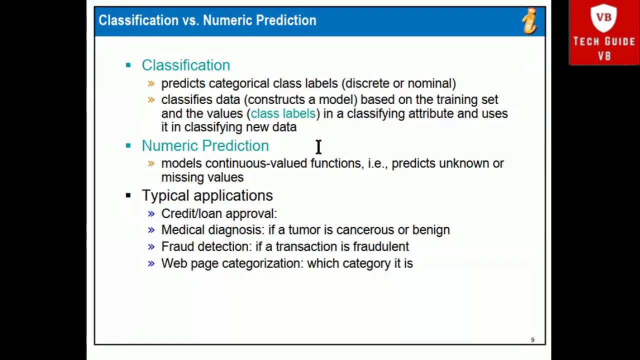 learning is basically used for the clustering. next we will see the classification versus numeric prediction, that is, classification versus prediction, as the term suggests. classification, what does it does the? it separates the labels, class labels. class labels are categorical. class label types is in two forms: descr ite or nominal. 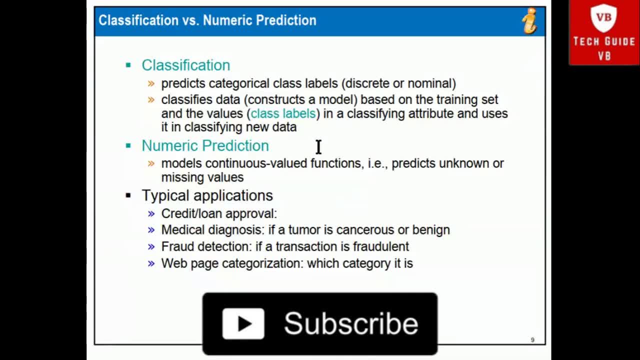 classifies data, that is, constructs a model based on the training set and the values, that is, the class labels in a classifying attribute and uses it in classifying new data. this is the classification, so according to the class, the data based on the training set and the values, and if the new data comes, 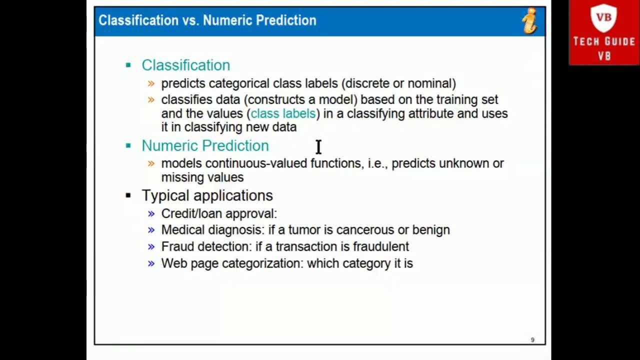 then what does what it does? it does the numeric prediction. so models continuous valued functions, that is, predicts unknown or missing values. so, according to the testing, if it does the prediction, but for the prediction there should be a training set. also, according to training set, it will train the model and it will. 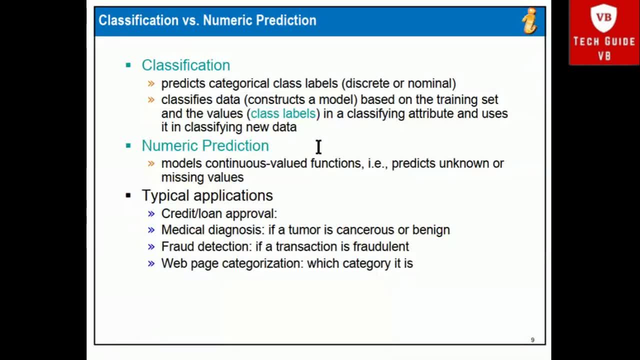 do the prediction based on the training set. so what are the typical applications of the classification or the predictions? the, the first, very important, is the credit or loan approval application. then the a medical applicationma Weise�� hebt bedijde ube vouscorole Anderson Germany. 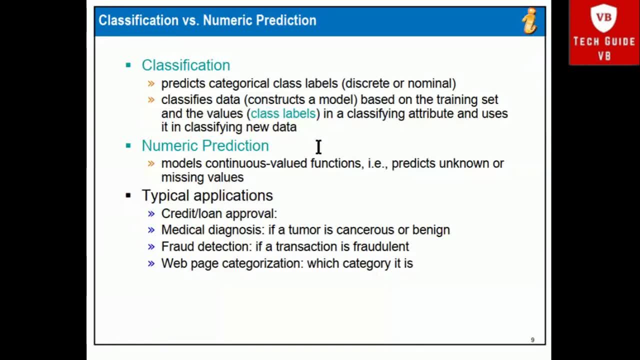 classifikasjaka prison creations. the. the first, very important, is the credit or loan approval application. then the medical diagnosis, for example, if a tumor is cancerous or not. then the fraud detection- if a transaction is fraudulent, and one of the application is the web page categorization- where which category it is that will be predicted with the. 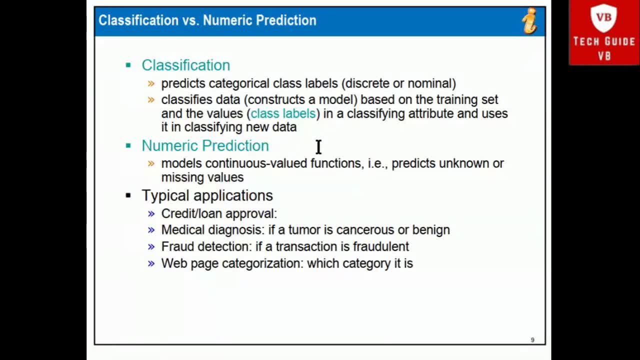 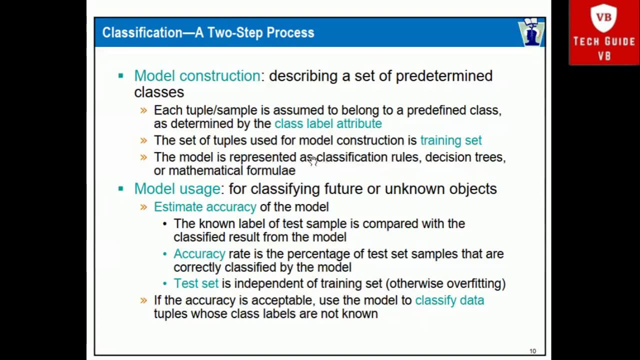 help of these applications. so these are some of the very important applications of classification. and then the classification, a two-step process, as I have told you, that the classification is divided into two parts: the training and testing. so the training is generally a model construction, where it describing a 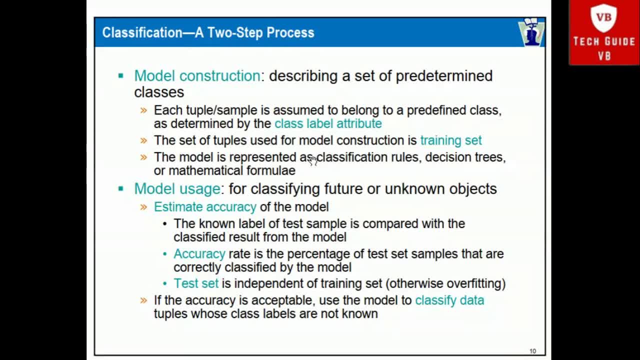 set of predefined, pre-determined classes. each tuple or sample is assumed to belong to a predefined class as determined by a class label attribute. the set of tuples used for the model construction is training set. the model is represented as a classification rule or decision trees or mathematical formula. so this is the model. 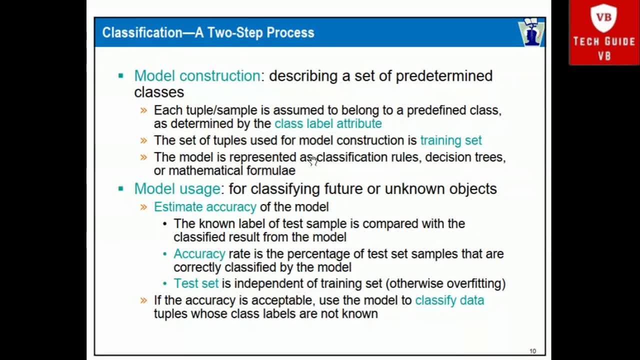 construction. there are different algorithms used for defining a model or for constructing a model. so, according to that, that algorithm training set is trained and the model is constructed, then the second step in this two step process is model usage. it is used for classifying future or unknown objects, that is, it uses 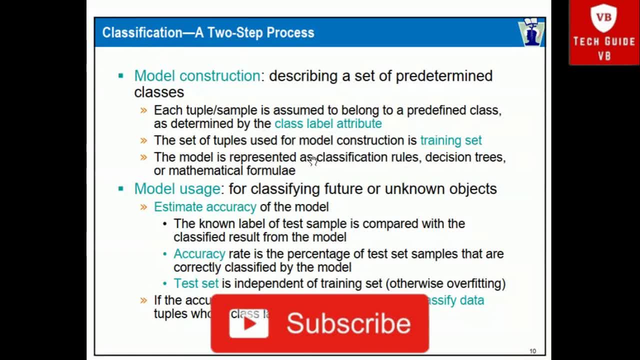 the testing set, that is, it estimate accuracy of the model, how accurate this model is. the known label of test sample is compared with the classified result from the model. accuracy rate is the percentage of the test set samples that are correctly classified by the model. test set is independent of training set. 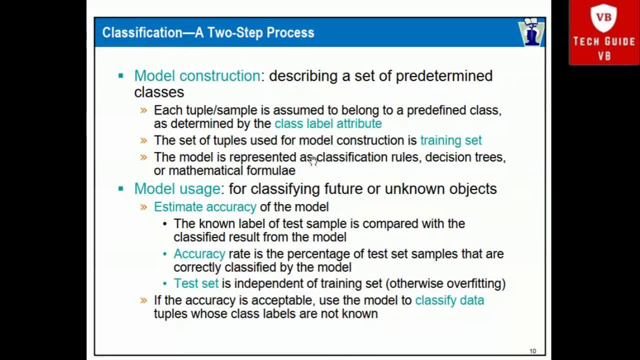 otherwise overfitting the accuracy is acceptable. use the model to classify data tuples whose class labels are not known. so I will give one very important and well-known example of stock market prediction. so in stock market, you know, every day there is a different value of the particular stock in the market. that value will go, or. 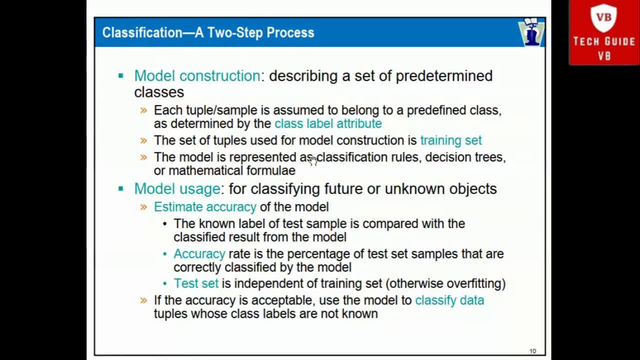 will lower. so we have the historical data and if you want to know the tomorrow's or day after tomorrow's stock value, particular stocks value, then what we will do, we will do a classification. so in this the model is constructed likewise we. we will take the, the. 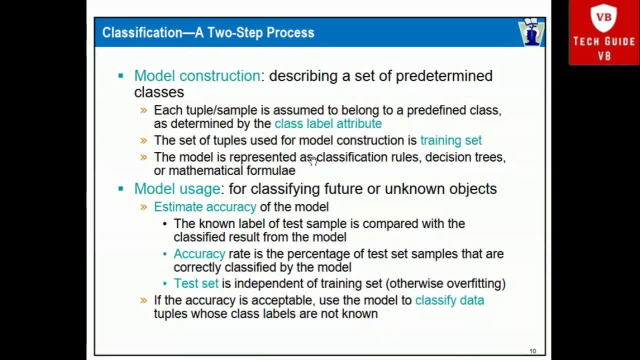 historical data, that is, previous days, particular stocks data, and we will construct the model according to that, using different algorithms. and if you want to predict the tomorrow's particular stocks value, then we will assume some of the value of tomorrow's and we will use the model which we have trained earlier, and then we 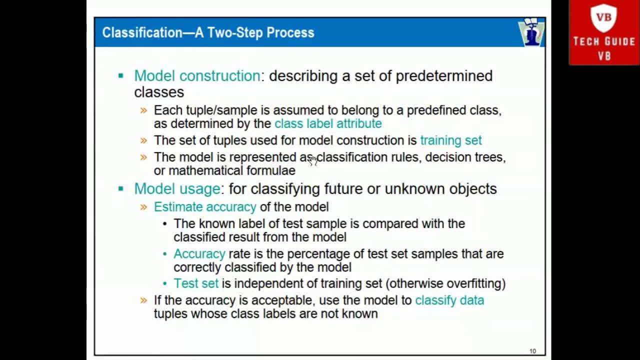 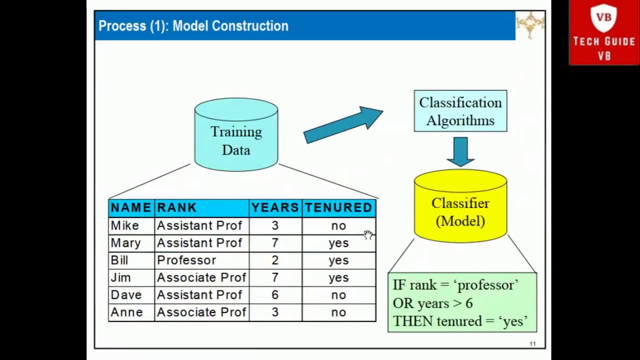 will get the result that whether this stock will go high or whether it will go low. so this is the two-step process of classification, then the diagram, material view and the another example is given here. the process one is model construction. as I have told, there is a training data. so 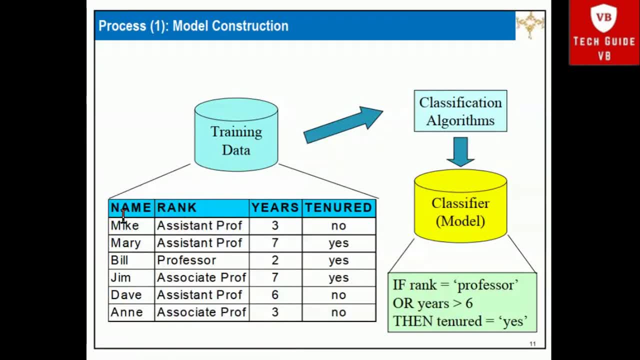 for this training. this table is given here. the mikk is a system professor and it has a. he has a experience of three years, so the result is no tenured. Mari is a system professor, have 7 years experience, so it has a. or should not be the result. of these trading data. it is not a ma leading balcony which is given by the which is given here. the mic is a system officer and it has a. he has a experience of 3 years, so the result is: note: annual married Boeghe options has b-1 years, so it. 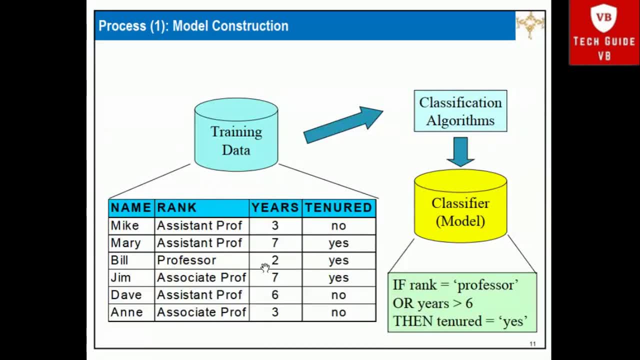 has a or she has a tenured. likewise, this data is given. so, according to this, what we will see here, we will use the classification algorithm, different classification algorithms and different classifiers and models, and this will give the formula that, that is, if rank is equal to professor or years experience. 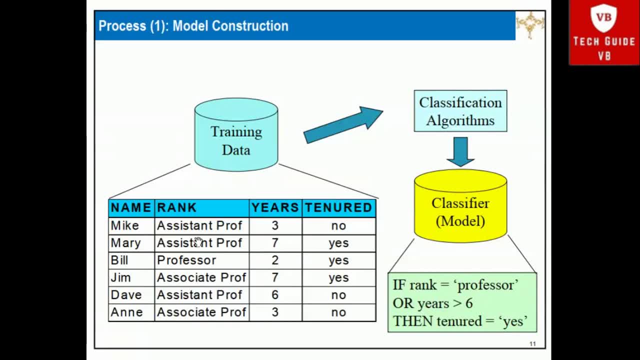 years are greater than six, then tenured is equal to years. see here the system: professor has the six or more years of experience has, yes, tenured. then the professor which has the two years of experience also has a tenured, yes, so the two conditions are here. rank is equal to professor or experience years. 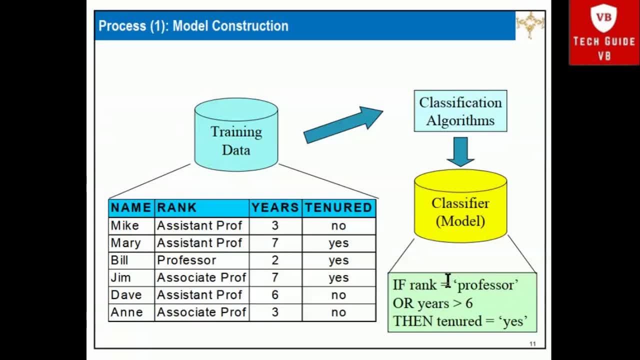 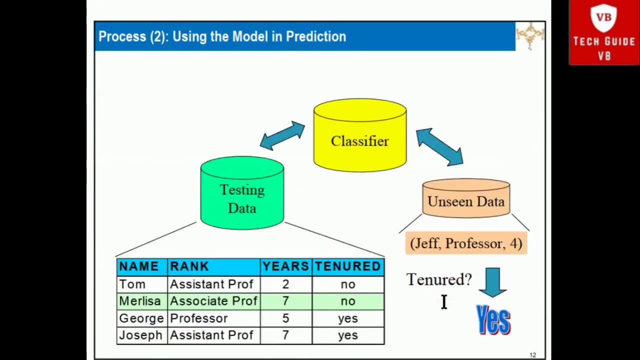 greater than six, then it will classify to yes tenured. otherwise it will classify to no tenured. then the second process is using the modeling prediction. we have trained the train the set using earlier table, so now we will just use the this model to predict some of the tenures. so 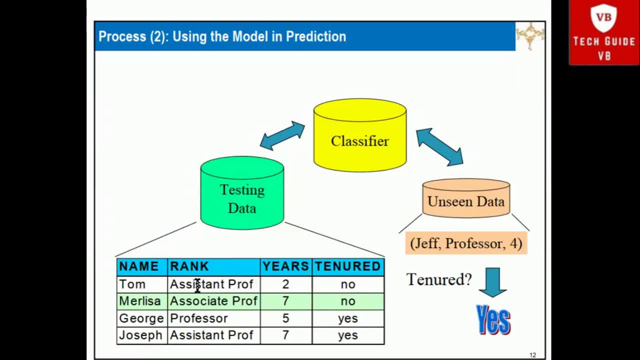 if new data is TAUM, which is a, a system professor and has experience of two years, then we will give the answer as no, because our formula is experience mode. if it is a assistant professor and I experience has six or more years, then tenured is yes, otherwise it is false. if professor, then 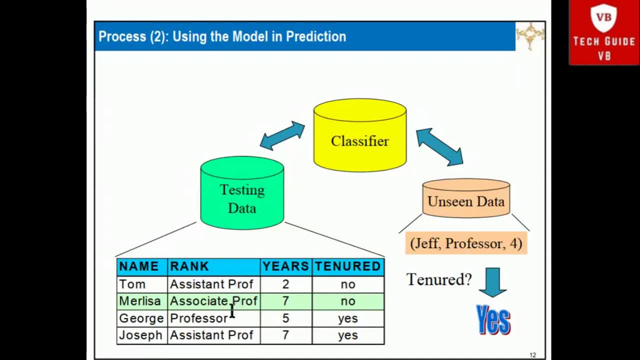 the tenured is yes, so this is predicted by our model. okay, but you can see here this prediction. second, records prediction is wrong here. so the accuracy of our model is 75% because out of four records, the three records prediction is correct, but the one record operation is wrong. okay, so 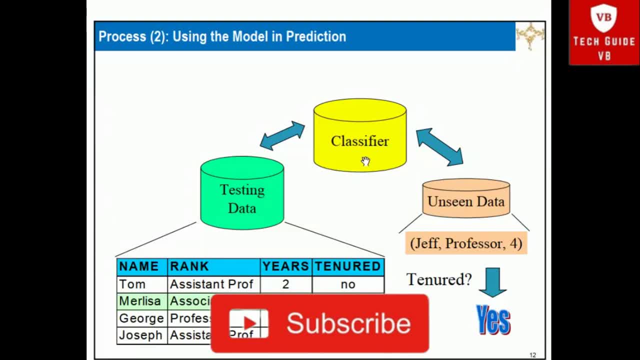 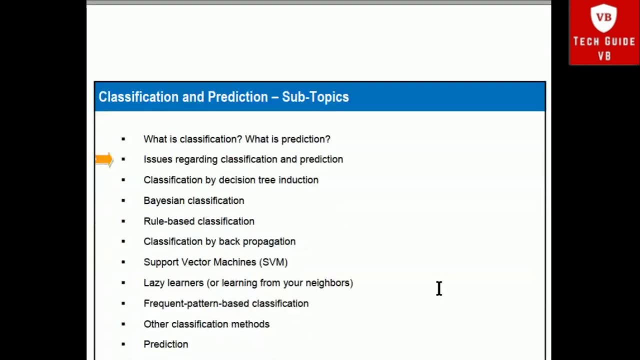 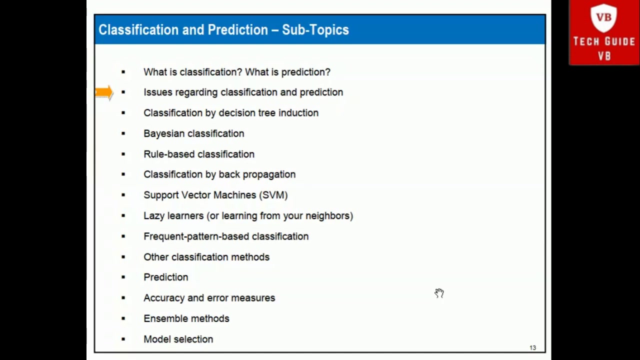 testing data is here according to classifier or the formula which we have constructed in earlier model. we will use this for unseen data and we will give the decision about the tenure here. okay, this is all about the what is prediction and what is classification. now we will discuss issues. 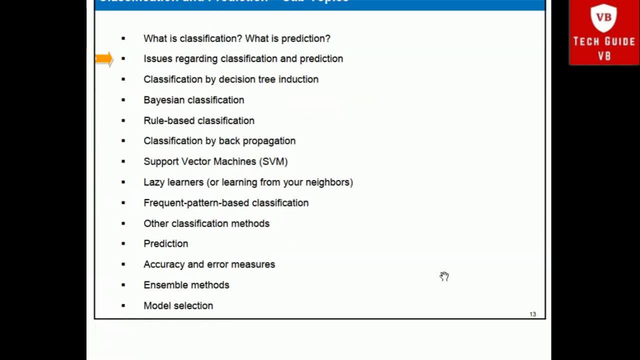 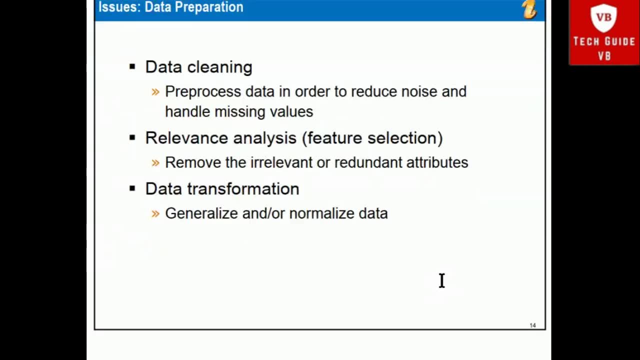 regarding classification and prediction. what are the different issues in classification, prediction? so the first issue generally is data preparation, where in data preparation, you know the data cleaning, relevance analysis, data transformation- this terms you have seen in earlier videos of this series- data mining and data mining concepts and techniques. if you don't know this term, then please do watch the earlier videos of this. 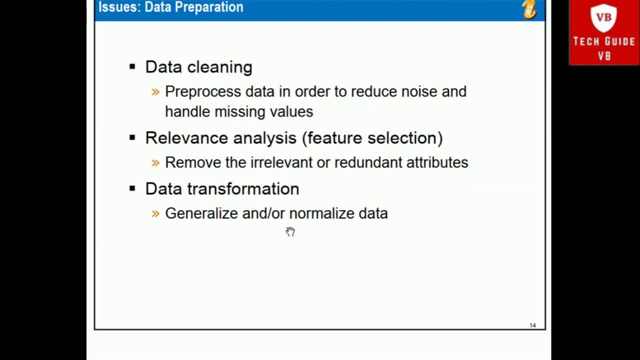 channel. okay, you will get to know all the terms in data cleaning it pre-process the data in order to reduce noise and handle missing values. so this will be a issue in data preparation. then the relevance analysis, which is also called as a feature selection, in removing the irrelevant or redundant attributes, this will give a issue, okay. 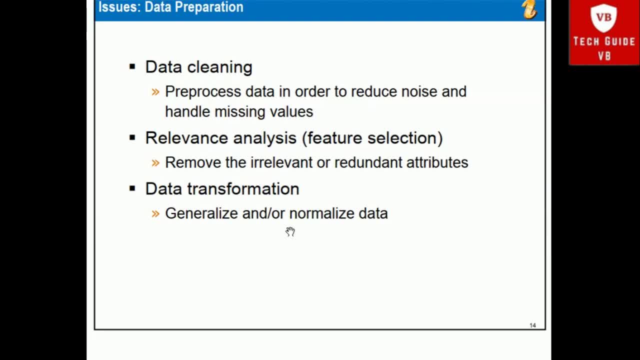 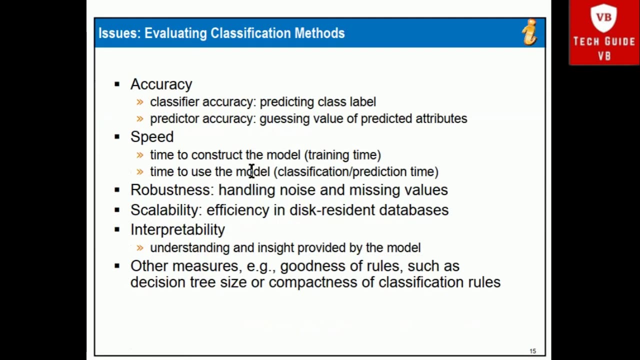 then the data transformation: the generalize and normalize the data. this may be a issue in data preparation. so these are the issues related to data preparation. then the: there will be a big issue in evaluating classification method: which method to use. this is the big question in the classification: how to evaluate this. 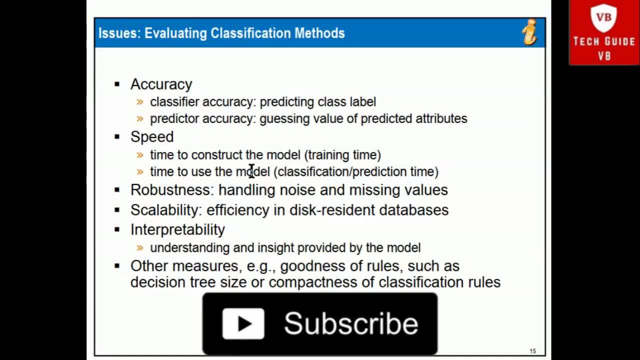 classification methods is the main issue. so, according to accuracy, according to speed, robustness, scalability, interoperablity and other measures, we will use this classification methods. so if bottoms-up ика, we consider the accuracy, classifier accuracy must be there or predictor accuracy must be there. what is classifier accuracy? predicting the class label is the classifier accuracy. so how correct? 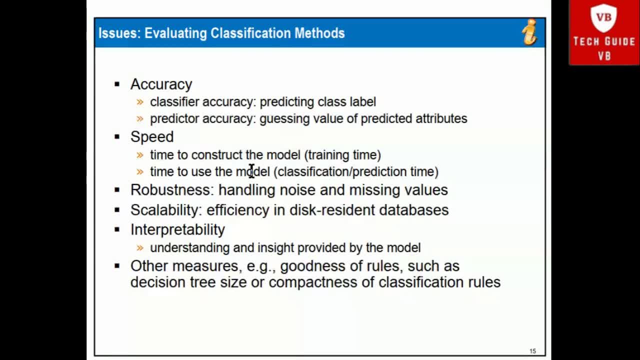 this model is predicting. the classifier accuracy is one of the issue. then the predictor accuracy is guessing the values of predictor attributes, so this is very important. then the next issue is speed, about the speed time to construct the model will be different for different models, so training time is one of the issue, then the time to use the model, that is, the execution time. 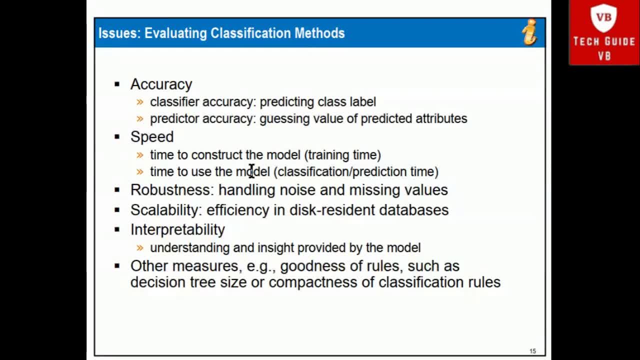 or prediction time is different in different examples. so this is the issue. then the robustness, that is, the handling, noise and missing values. this will be a issue. then the scalability: if we take the example of scalability, there is a issue in efficiency in disk resident databases. so if we scale up our system, then the storage problem will be there. so this is the issue. 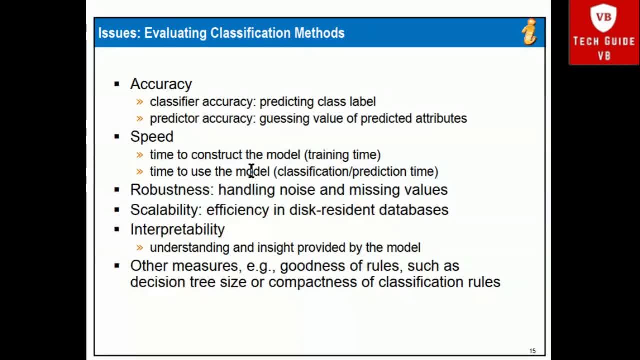 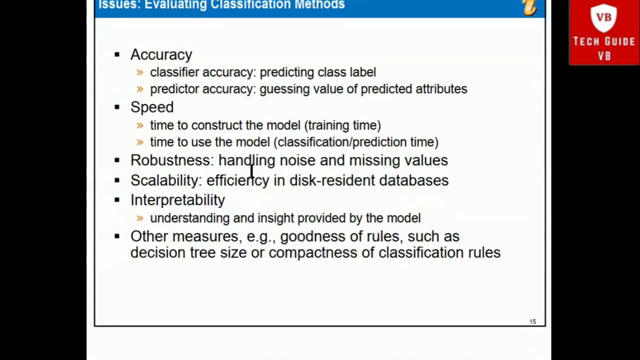 then the interoperability, that is, understanding and insight provided by the model and other measures, are goodness of rules. let us introduce some more concepts, which calls citation training, such as the decision 3, size or compactness of classification rules will be there. now we will see the classification by chance 3, induction. 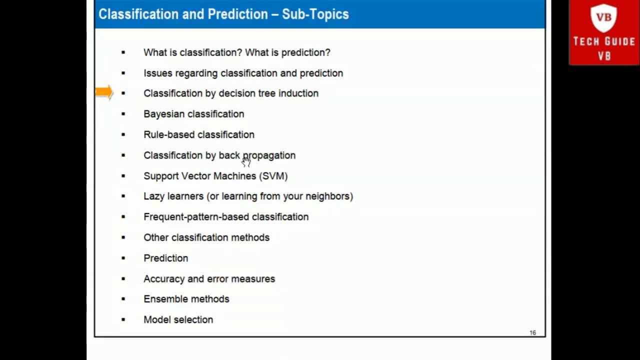 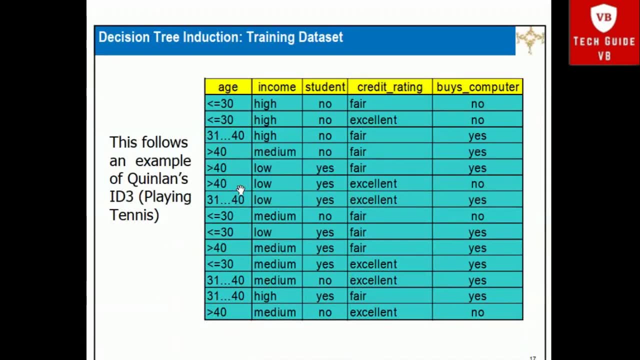 so the decision 3 induction is 1 of theนะคะ to use further classification of generation 2 lien collection. we will take this training data set, that is, the historical and artificial data set, donné home data set to grade the number of points up within the哦. this will shall know in different aspects that the this is the Mill школing, so that this uh is which we can two or be the Roots ovenization has. We'll take this shilling data set to grade the coû sud cap andamientos in terms ofρεί as four, or it will be 13. 16.. 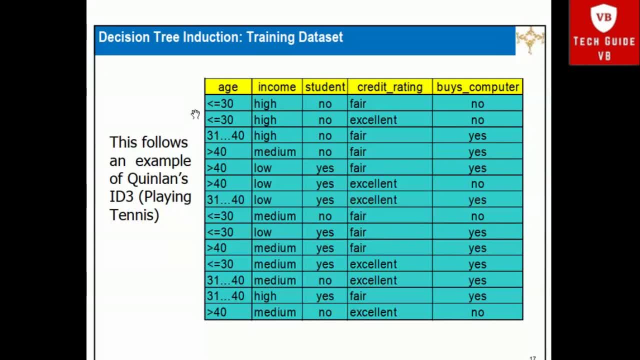 data which we have got. this follows an example of Kunlans ID 3 that is playing tennis. so if age is greater than or less than equal to 30, income is high and if he is an, he is not student and credit rating is fair, then whether he will buy. 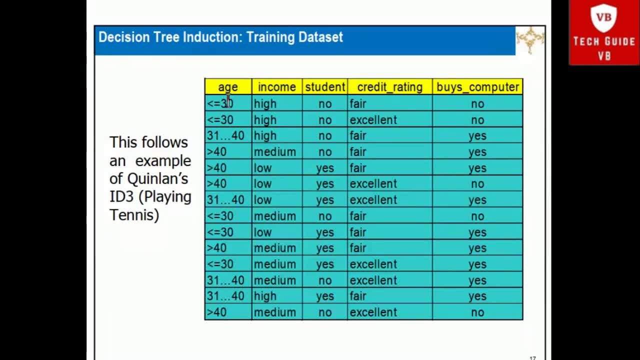 a computer? no, he will not buy a computer. when he will buy a computer, his age is between 31 to 40, income is high, he is not a student and credit rating is fair. then he will buy a computer. this is the training data set which we have taken. 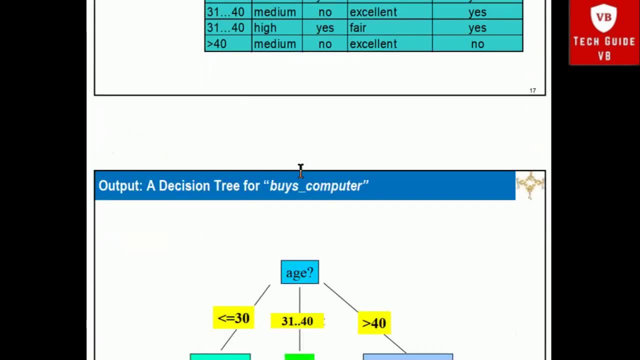 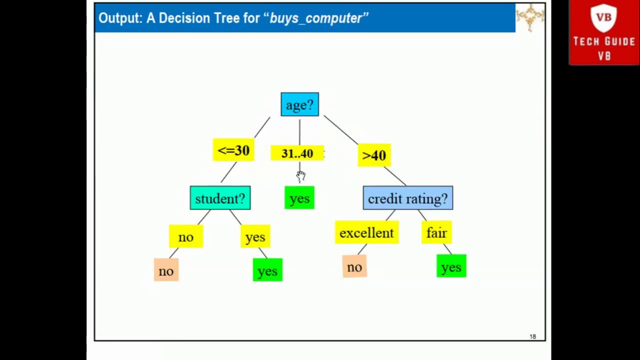 and we will train our model according to what we want to find a decision tree for: buys a computer, whether that person will buy a computer or not. so, according to the table which we have seen earlier, this is the diagram for this decision tree, that is, if age is less than equal to 30 and he is a student. 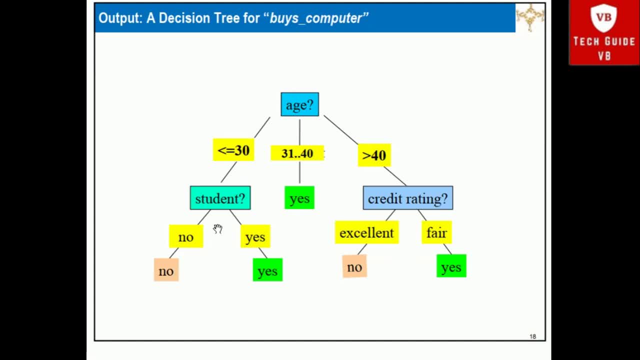 and if it is not, then he will not by a computer. he is a student, then yes, he will surely buy a computer, because student needs a computer or laptop for their study purpose, then if the age is about in between 31 to 40, then he will surely. 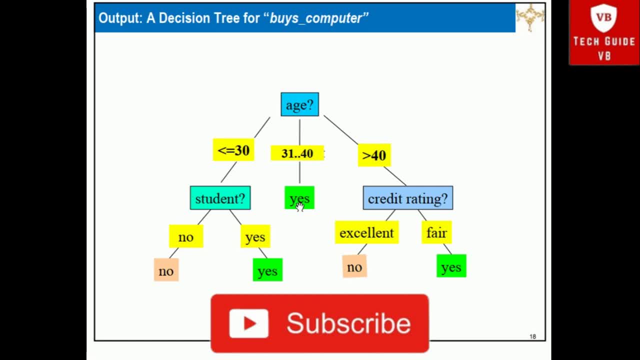 buy computer. if the age is greater than 40, then there will be a different criteria whether he will buy a computer or not. if the age is greater than 40, credit rating is excellent, then he will not buy a computer. if the credit rating is for fair, then surely he will buy a computer. so this is a decision. now the algorithm. 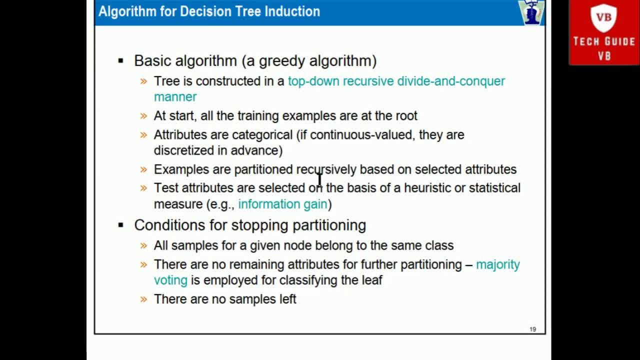 for decision tree induction. the basic algorithm is based on the greedy algorithm. okay, really is very well known algorithm. at start all the training examples are at the root. attributes are categorized, that is, if continuous valued, then they are discretized in advance. example: our partition is recursively based on the selected attributes. test attributes are selected on on the basis. 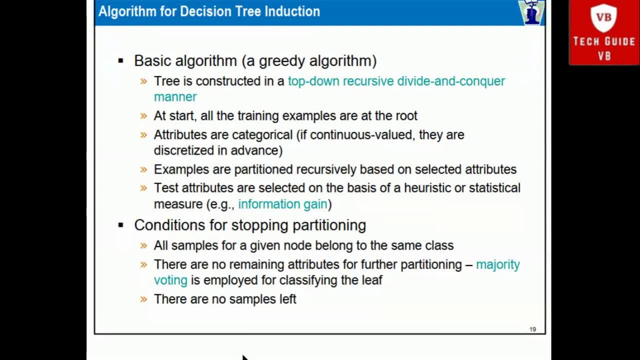 of historic, heuristic or statistical measures. this is the basic algorithm for this decision tree induction. that is for a greedy algorithm. so basically a top-down approach, that is, the divide-and-conquer manner, is used in this algorithm. then the water condition for stopping partitioning: all samples for a given node belong to the same class, then the partition will be. 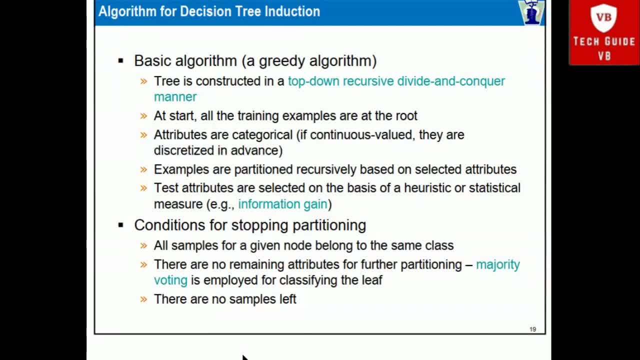 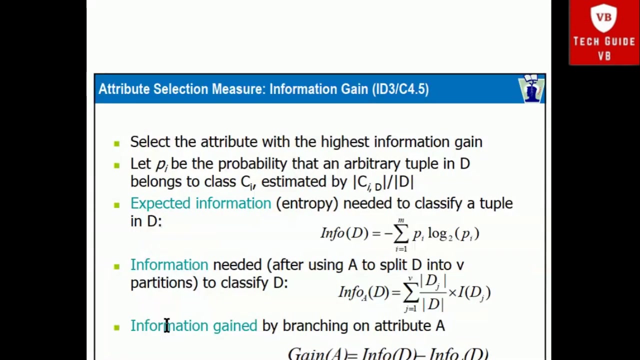 stopped. the second condition is there are no remaining attributes for further partitioning, that is, the majority voting is in employed for classifying the leaf and there are no samples left. in that three conditions, there will be a stopping partitioning or partitioning will be stopped in these three selection measures. that is the information gain in. 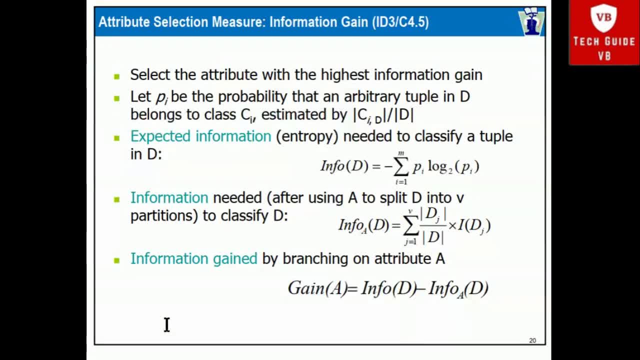 this does, it will select the attribute with the highest information gain. let P be the probability that an arbitrary tuple in D belongs to class CI. estimated by CID divided by D, the expected information is needed to classify a tuple in D. the formula is given here, which uses the log. 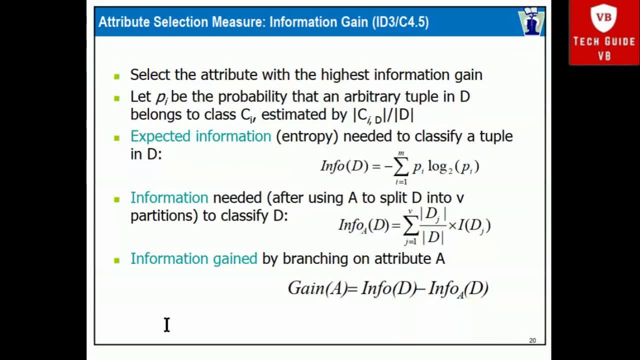 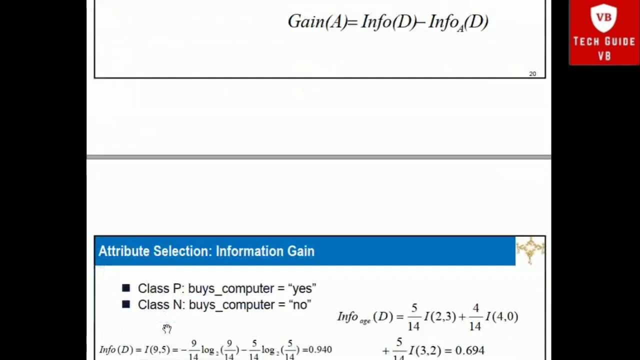 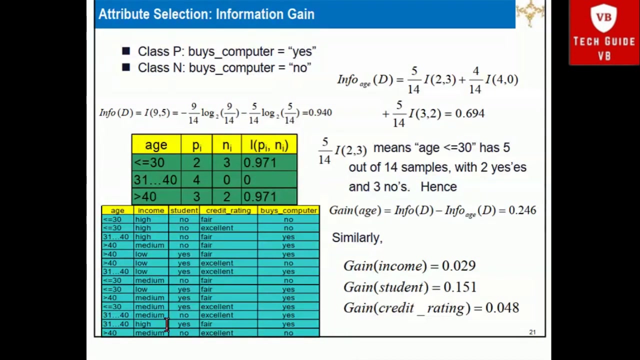 in mathematics, then the information needed to classify D is: after using a to split D into V partitions: ok, the formula is given here. then the information gained by a branching on attribute a, that is gain. a is equal to info, D minus info. da now the attribute selection, information gain. 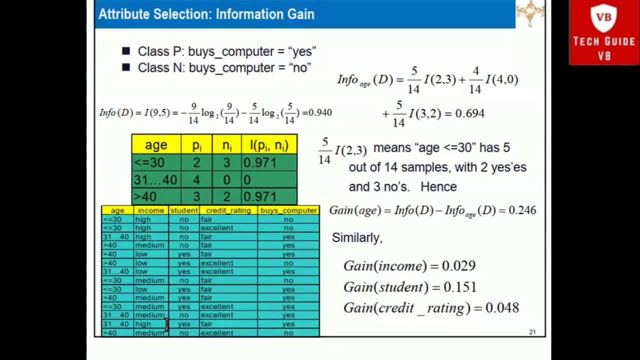 class P buys computer. yes, it buys a computer. class N did not buy a computer or will not buy a computer. so how we will decide that? so, according to the historical data, we will train the model and according to training of model, we will use this training set for testing purpose and for the. 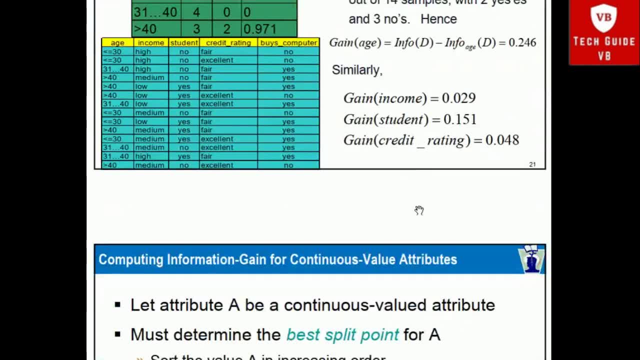 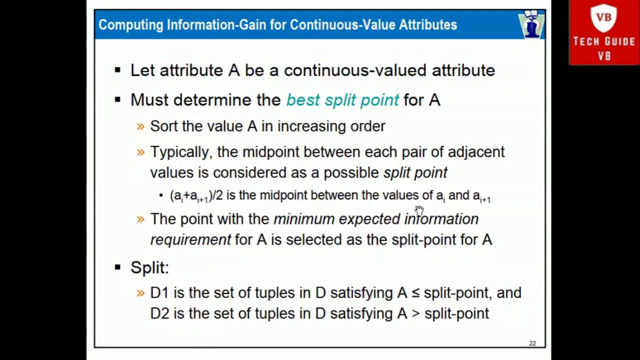 prediction computing information gain for continuous value attributes. let attribute A be a continuous valued attribute and must determine the best split point for A and B, that is, it sorts the value A in increasing order. typically, the midpoint between each pair of adjacent values is considered as a possible split. 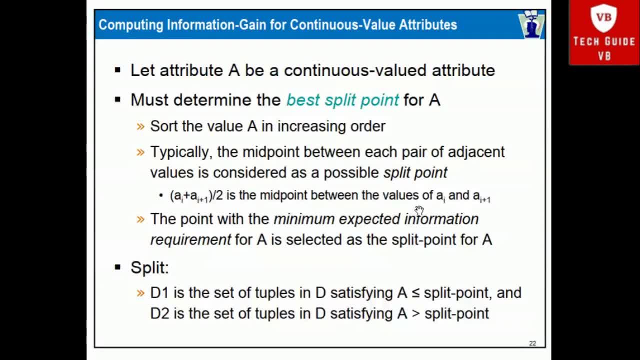 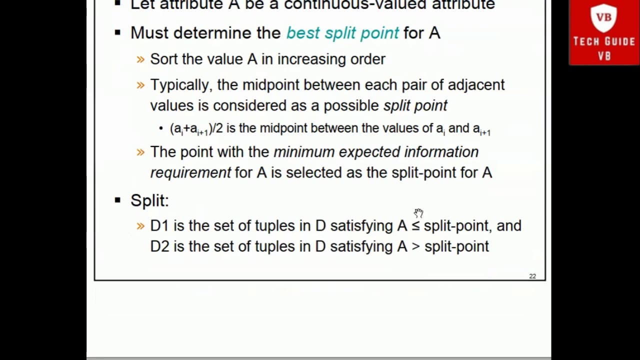 point and is the midpoint between the values of AI and AI plus 1. the point with the minimum expected information requirement is that the midpoint of A is selected as the split point for A. the split D1 is the set of tuples in D satisfying A less than equal to split point. 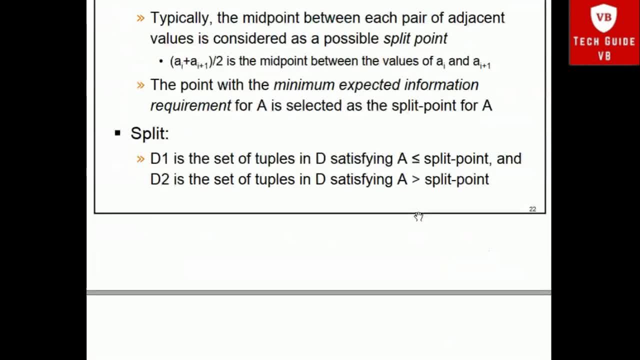 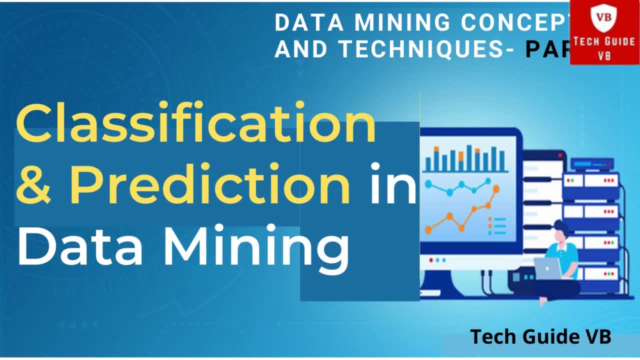 and D2 is the set of tuples in D satisfying A greater than split point. specification and prediction. ok, subtopics which we have covered are basically three: what is classification, what is prediction and what are the issues in classification and prediction? then we have seen the decision tree. 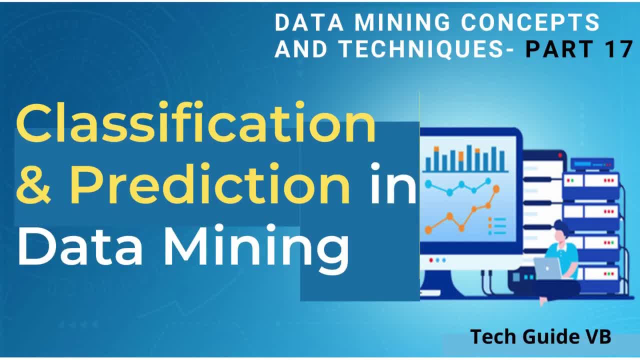 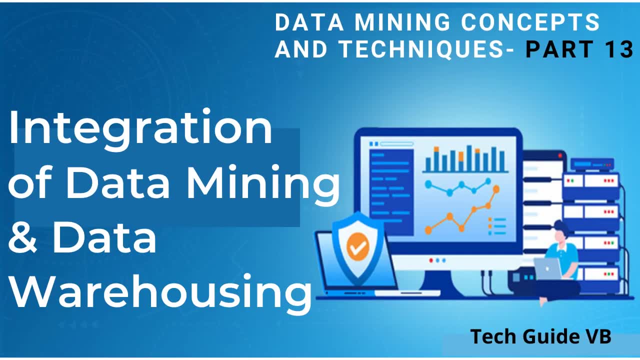 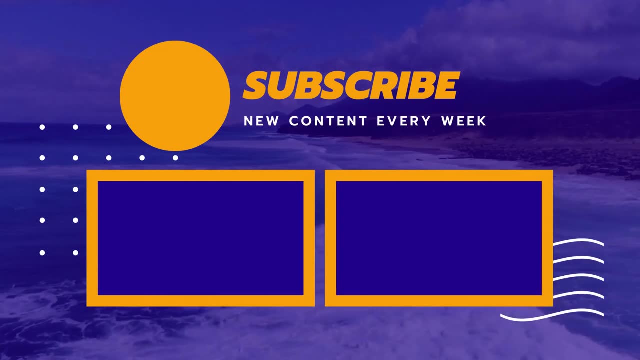 induction, basically. so this is all about today's video. do like, comment and share this video to your friends. if you are new to the channel, please do subscribe to channel. for latest updates, press the bell icon and keep learning. keep watching. thank you, Jai Hind.